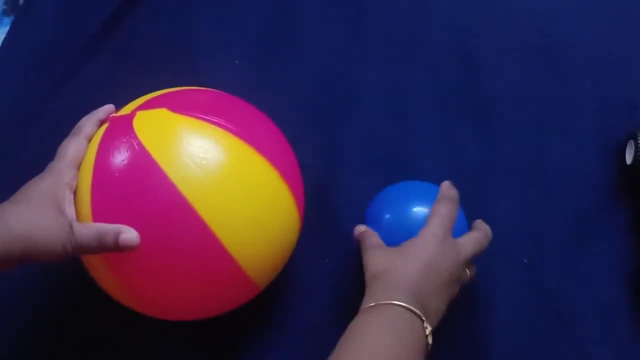 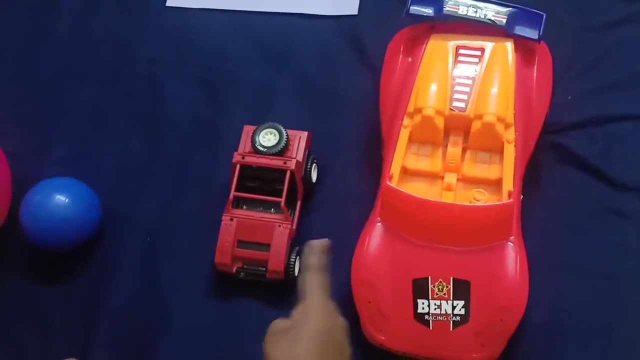 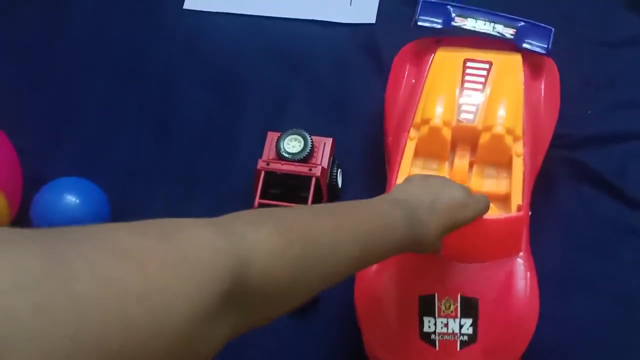 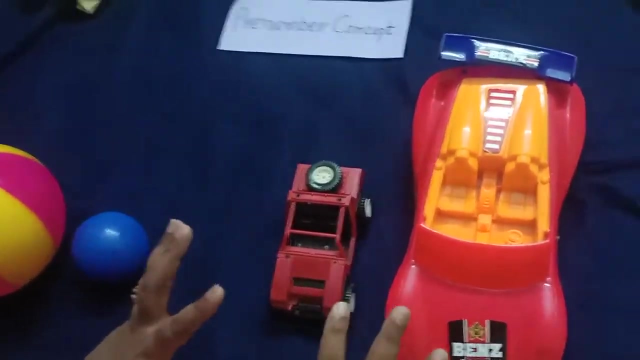 this is big, This is small. Okay, now I'll show you one more example. So see, here I have two cars. Can you able to see the sizes of this car? This is a small car And this is a big car. Okay, now can you able to differentiate big and small? Okay, now ma'am is going to show you the heavy and light. Okay, children, the next one we are going to learn is heavy and light. 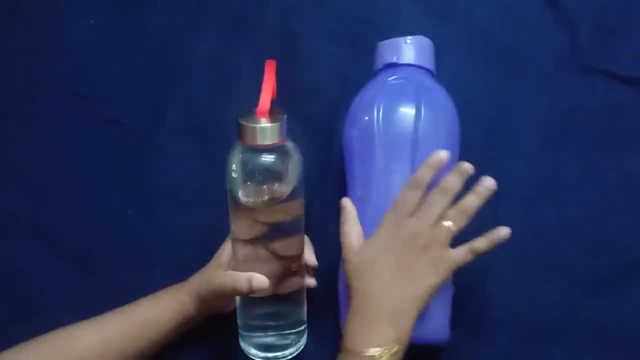 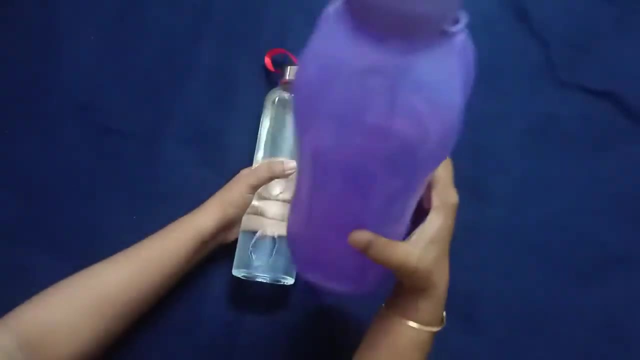 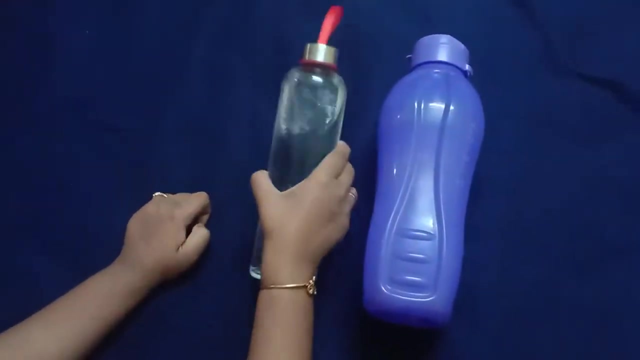 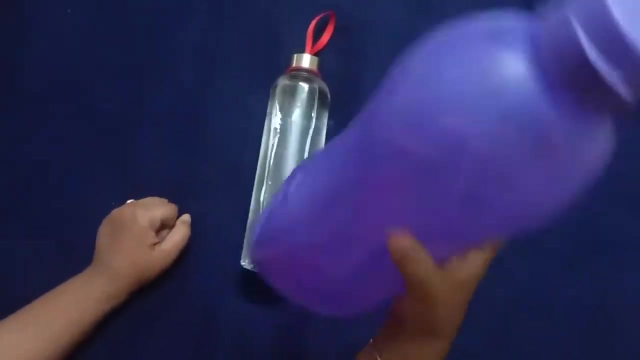 You know what is heavy? See, here I am having two water bottles. This water bottle I have filled with water, So this water bottle having water And this bottle is not having a water. So when I am lifting it, see, when I am lifting this, this is so heavy. Yes, because it is filled with water, But when I lift this, it is so light. You know why? Because this bottle is empty. 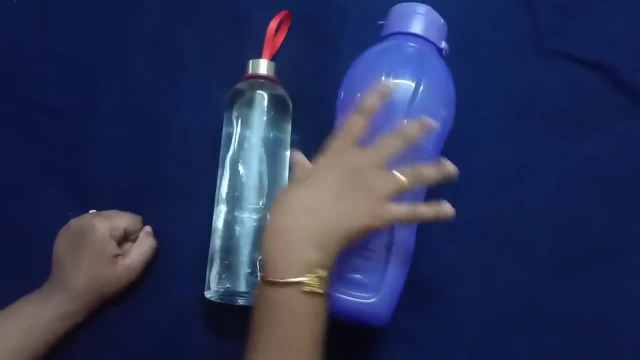 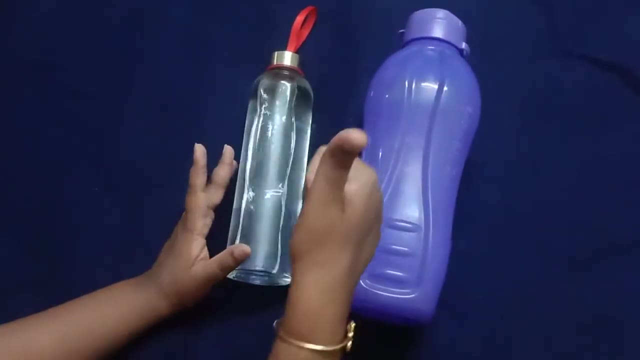 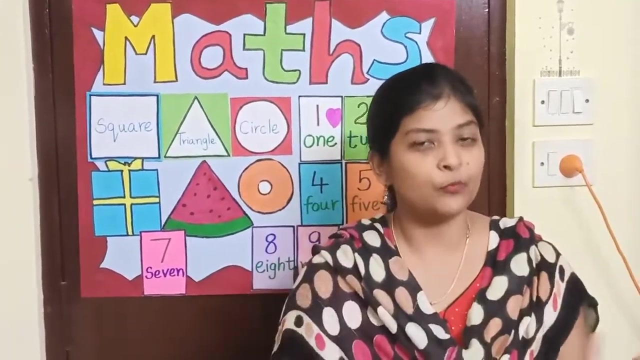 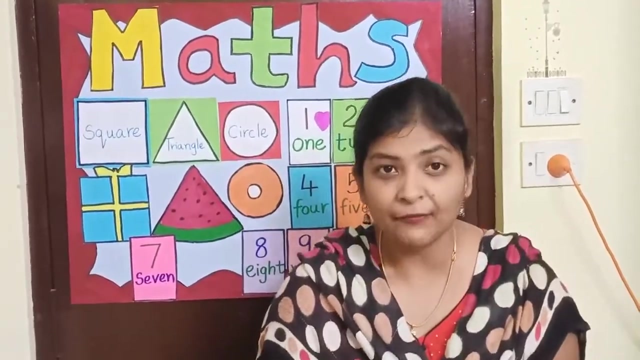 This is heavy because it is having water And it is light because it doesn't have a water. So this is heavy and light. Okay, children, Okay children. so what did we have learned today? Today, we have learned pre-number concepts. What we have learned, We have learned pre-number concepts. So, in pre-number concepts, what we have learned, We have learned: long shot, tall shot, big, small shot, big shot. 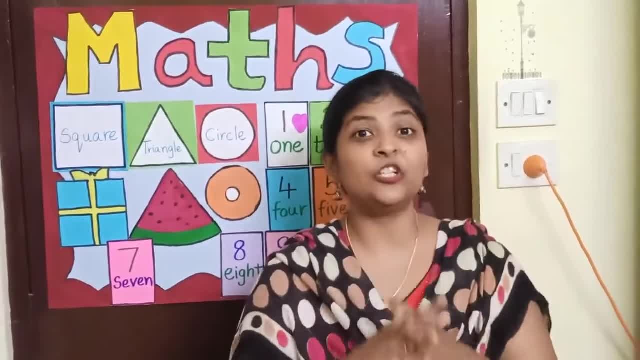 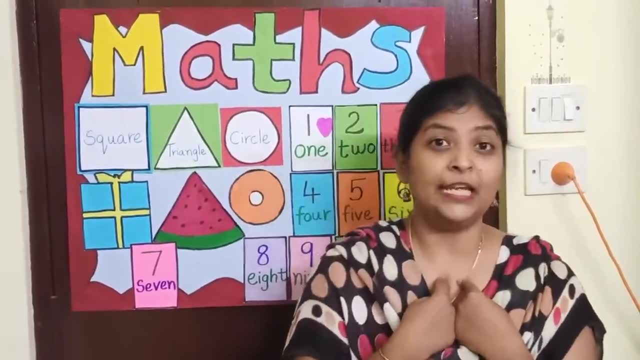 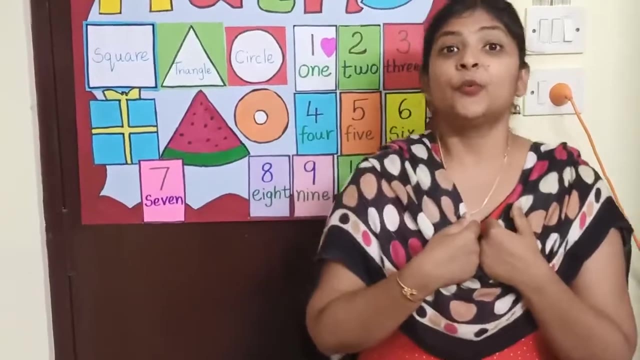 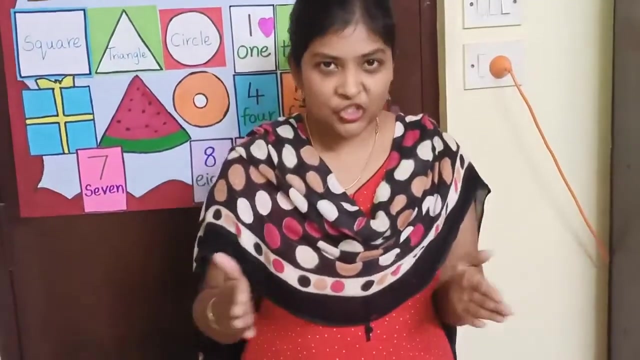 Small heavy light. Right Now ma'am is going to teach you with the action. Okay, So what you all have to do, you know you have to see ma'am nicely and you have to see how ma'am is doing the action, And then you all have to try with me. Okay, So when ma'am says long, you have to do like this Long shot. Long means you have to do like this Long shot. 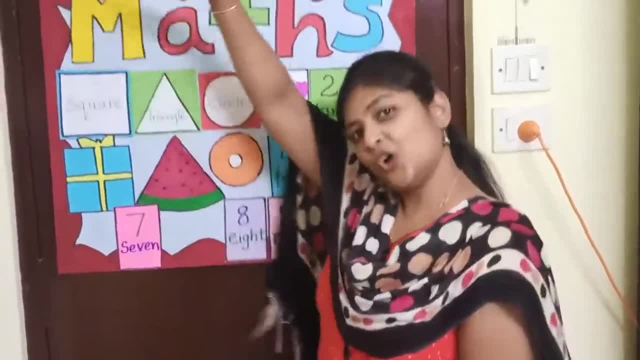 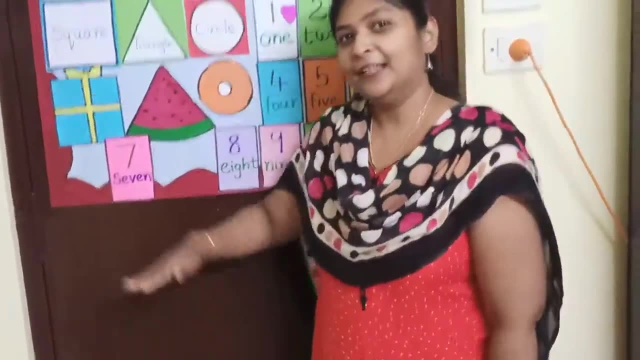 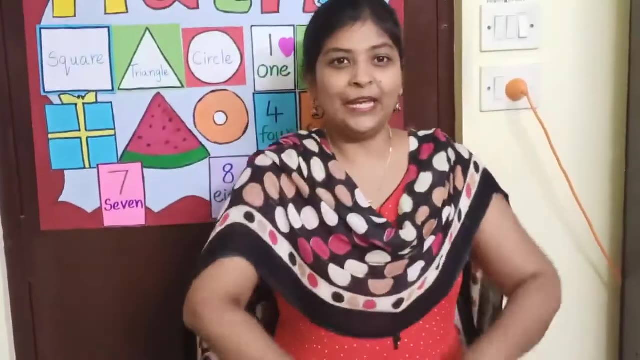 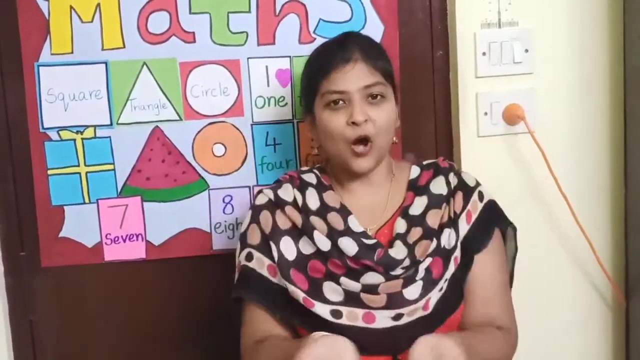 Long shot. Tall tall means you have to raise your hand up. Tall shot, Bend, Tall shot. Tall shot Now, big, Big, small, Big, small Big means you have to take the hands outside, So bigger. 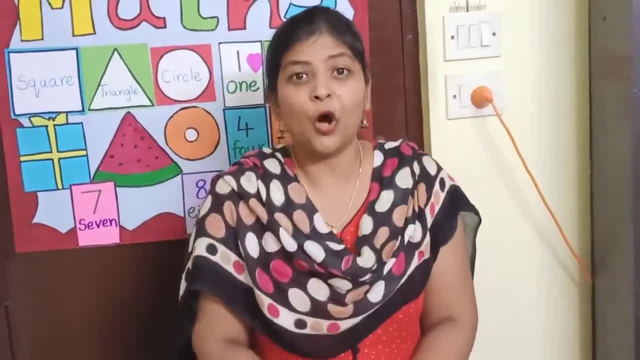 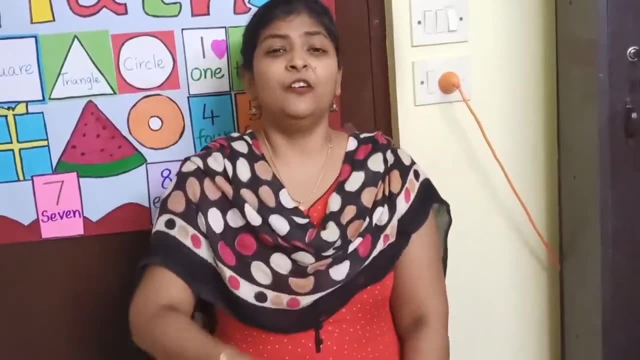 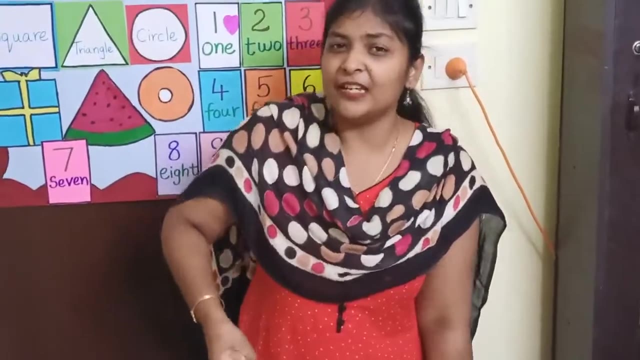 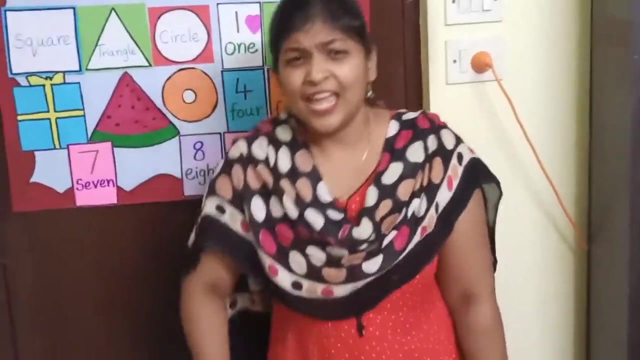 You have to make a big circle. Big Now small means small circle, Small, Big, Small Now heavy. When you carry a heavy thing, how you will feel: Heavy, Heavy, Heavy Light, Heavy Light, Heavy Light. 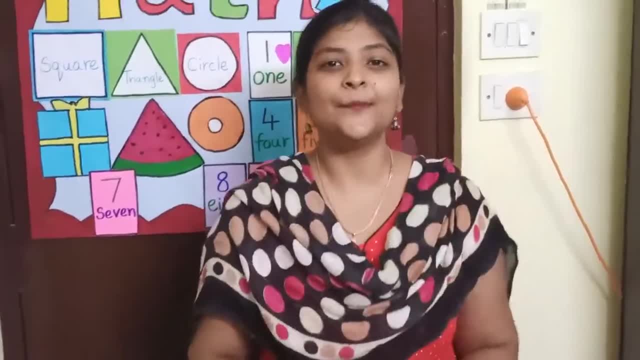 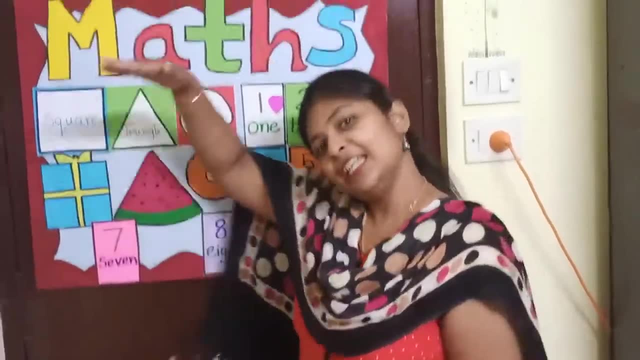 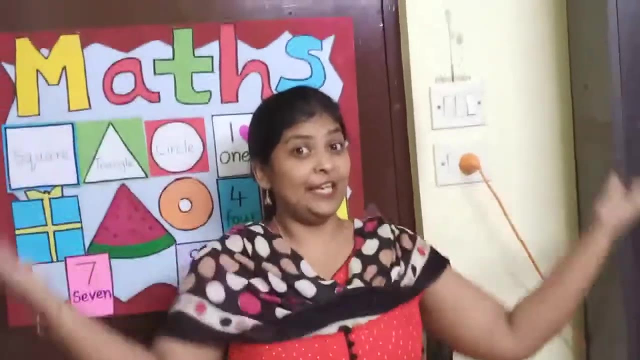 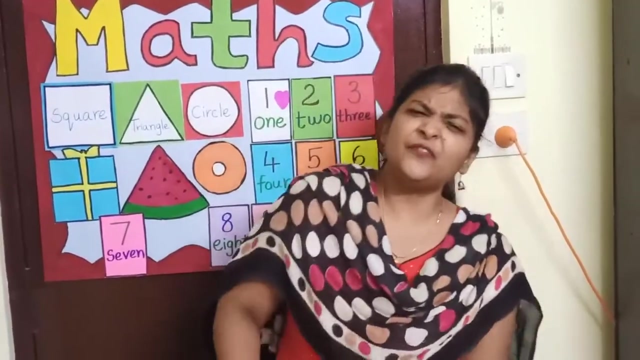 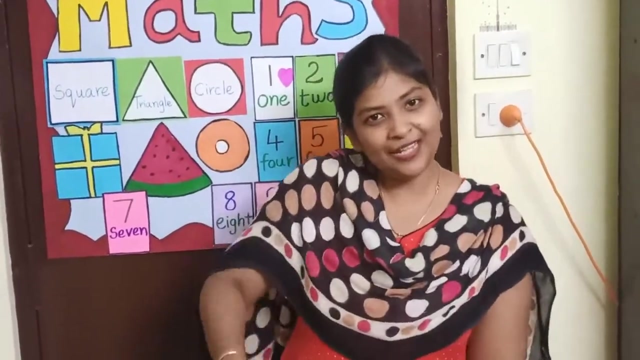 Now shall we do one more time. Okay, Long shot, Long shot, Tall shot, Tall shot, Big small, Big, small, Heavy. I am not able to carry it. It is so heavy, Heavy, light. Oh, it is so light. 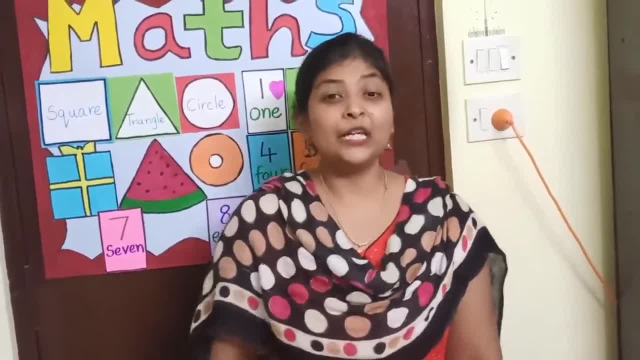 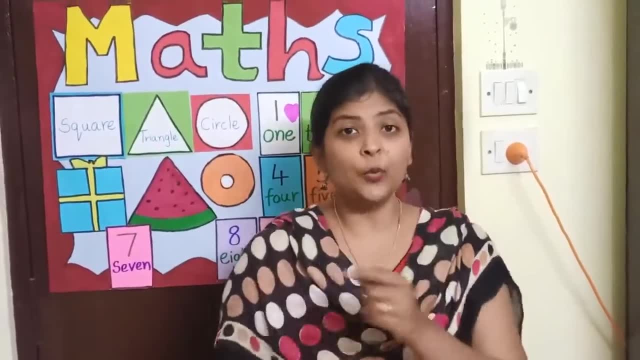 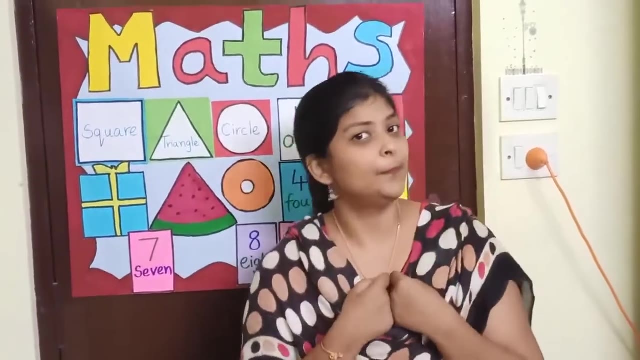 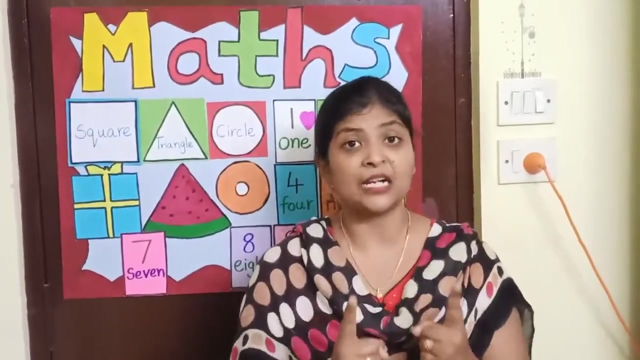 Heavy light. Okay, So practice this with the action and also practice in your home. Do your worksheet and try to finish all the worksheet by Friday, and you all have to send it to ma'am. Okay, Ma'am wants to see all your worksheets. Then only ma'am can able to put you marks. You all want to start right. So what you have to do: You have to do your worksheet and you have to send it to ma'am. Okay, 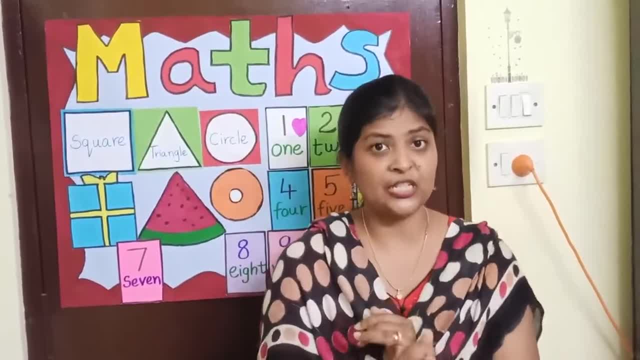 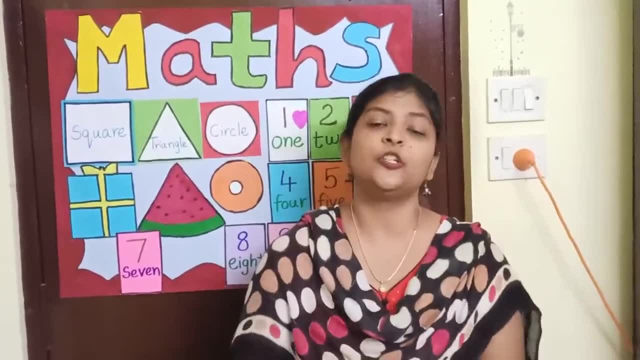 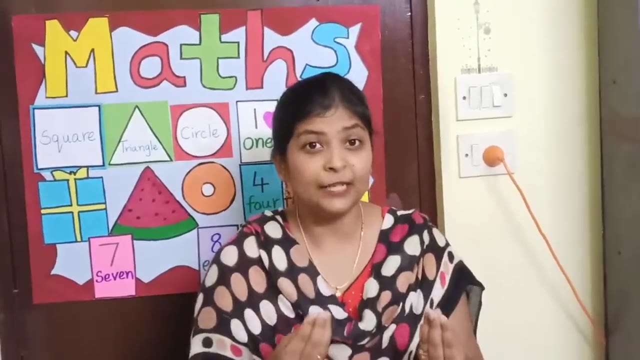 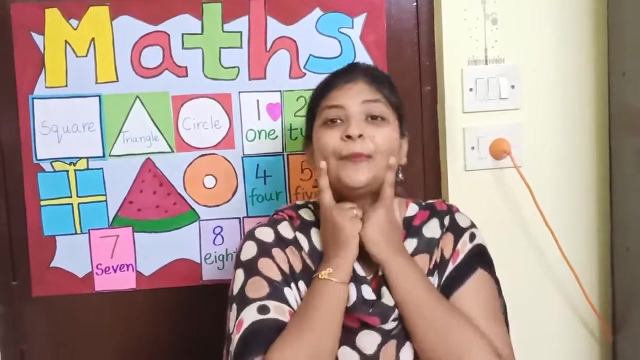 So Monday, I hope you all have finished your English worksheet and today you are going to do the math worksheet. So after finishing it, on Friday, the EBS worksheet, you can send it to us. Okay, children, Take care of yourself. Drink lots of water, Eat a healthy food. Don't eat junk food. Eat a healthy food, Obey your parents and always be happy. Always have smile on your face. When somebody sees you, you have to smile at them. 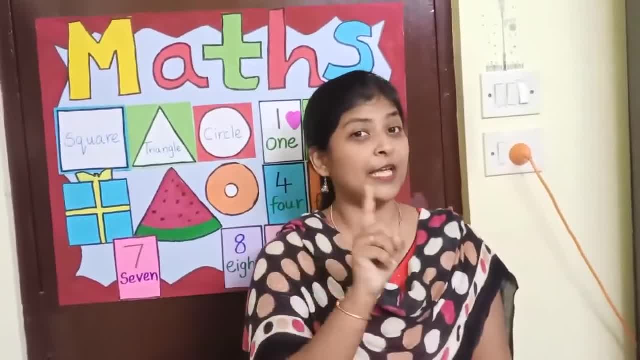 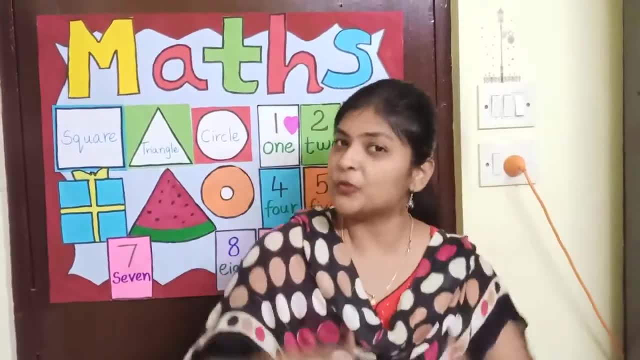 Okay, And the most important thing, don't forget to say the thank you prayer to God. I hope you all are doing it. If you are not doing it, no problem. From today onwards you can start doing it. Okay, Okay, children, take care, Bye, bye.